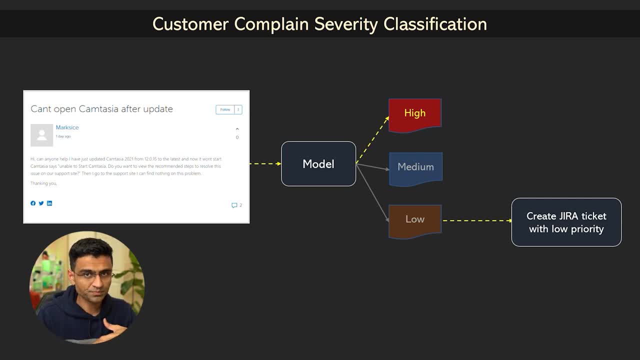 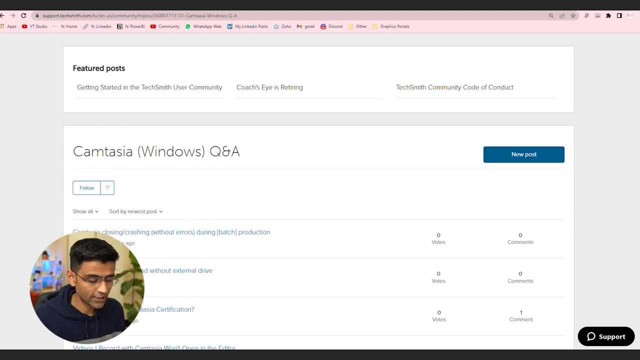 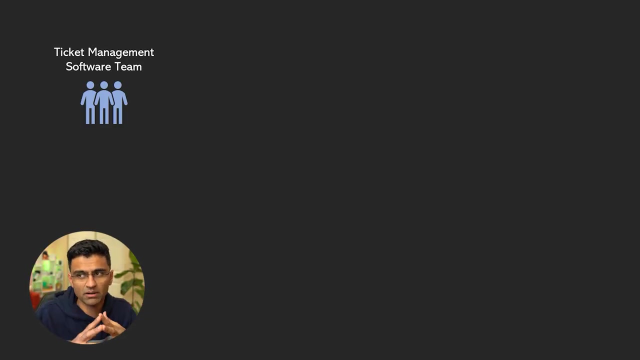 in Camtasia is using to create the ticket so that it doesn't require immediate attention but it can be looked on at some point in time. So now this particular module on Camtasia's website, let's call it ticket management system. It is created by some team in Camtasia. Camtasia, you know it's a software owned. 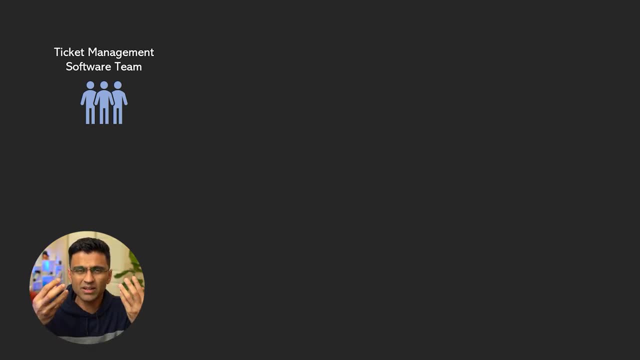 by TechSmith, and TechSmith company will have some software team which has created this ticket management system and they might be storing all the support ticket data in some database. Let's say that database is MongoDB, It could be MySQL or it could be NoSQL database such as MongoDB And these 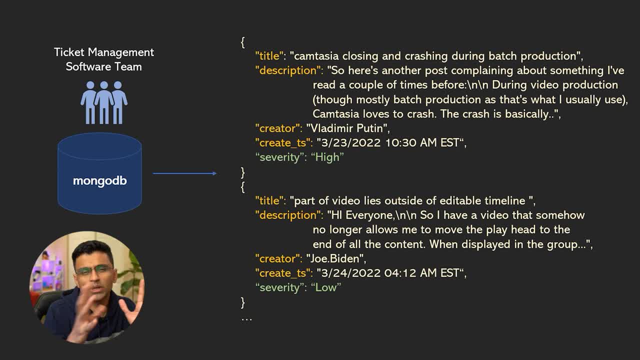 database will have all the ticket records. So I have shown two different tickets here in JSON format. This is a popular JSON format where you can have different fields of the ticket, such as ticket description, creator- Here it is creator timestamp, you know TS. 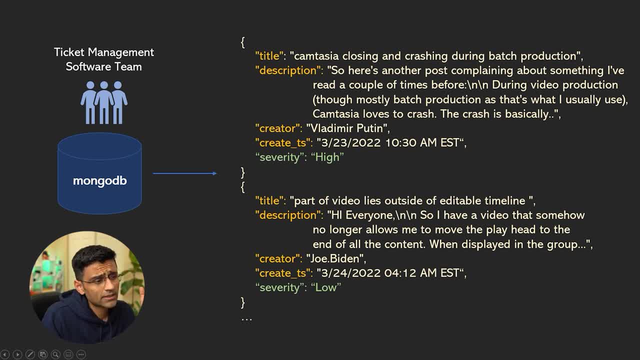 means timestamp, And you can have all these records in MongoDB and also watch this green field CVR ID. So let's say Camtasia has been running for five, seven years and we have already 10,000 tickets in our system. That's like historical data that we already have. 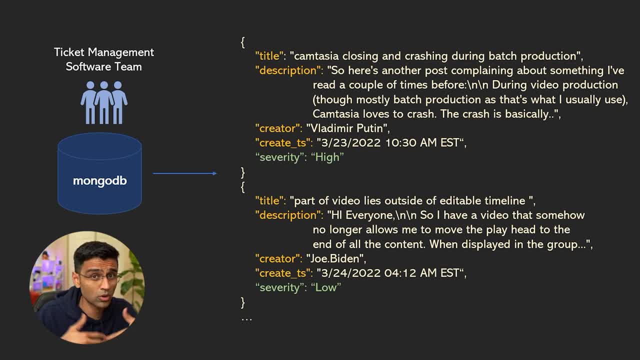 Now someone would have tagged those tickets as high or low or medium priority. So we have- let's assume we have- those labels. So this CVR ID- high, low- means we have the training data set that tells you if the description is something like this, then it's a high priority ticket. Sometimes you might not have these. 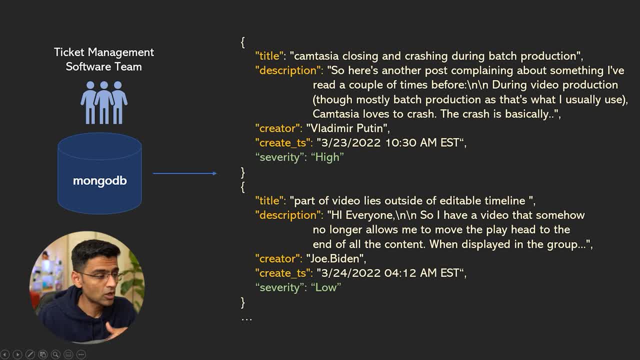 tags and you might have to hire human annotators to kind of go over the tickets and tag them as a high, low or medium priority. But for simplicity, we are assuming we have all this information. Now what happens? What happens is: in TechSmith company, there is an AI team or NLP team or data science team. 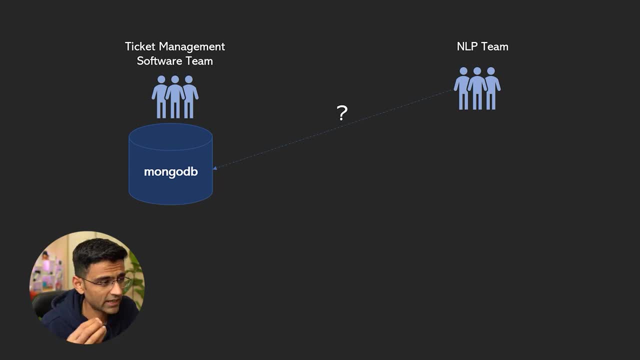 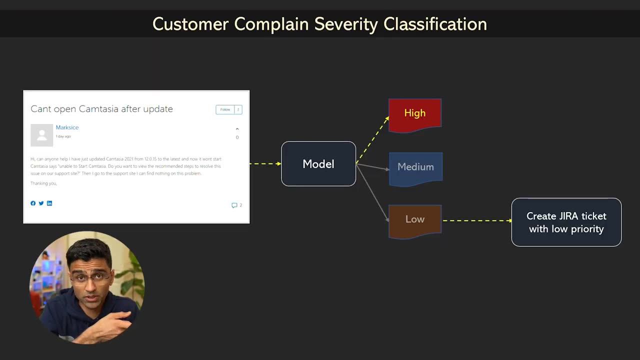 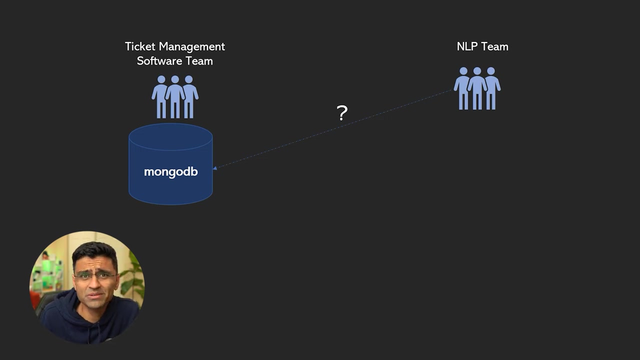 You can call it anything. And let's say, this AI team wants to build this particular model that I showed you here, And in order to build this model, they need all this training data. So they will go to ticket management software team and say, Hey, can you give me access? 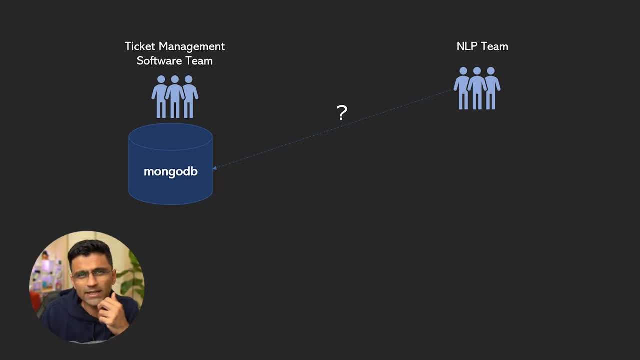 of your MongoDB And ticket management system might be like. we don't want to give you a direct access of our database. Maybe we can upload all our data to some cloud location, Let's say some Amazon S3 bucket. S3 is like a secure object store on cloud. 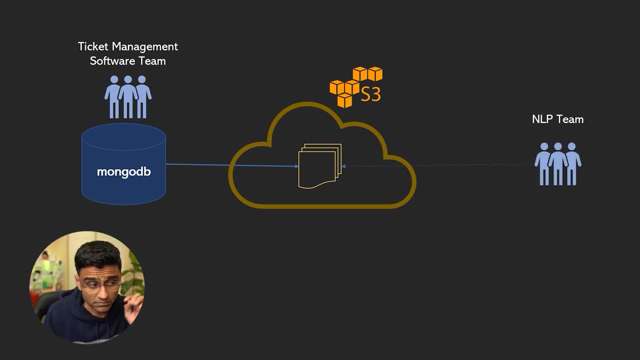 And we can push all the records there And maybe from there you can consume that information And build your model. Sometimes people build data warehouse also okay, so that their mission critical database is not impacted, And this step is called data acquisition. 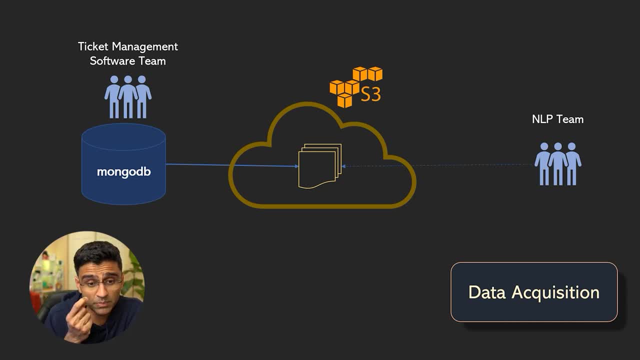 So data acquisition is a first step in NLP pipeline that is performed by NLP team And the idea here is to get necessary data required to solve a given NLP problem. Now here I gave a very simple example. Sometimes, when you build NLP team, you don't have training data set available. 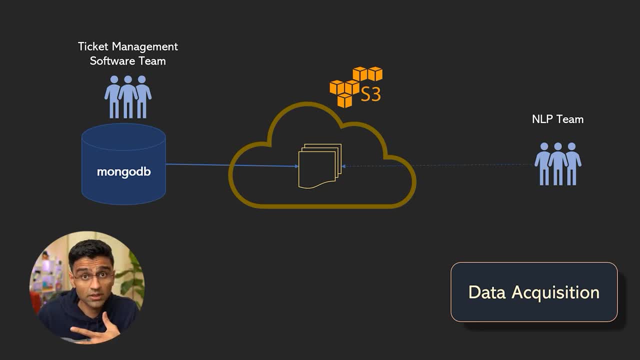 In that case you can use some external database, some public data set- there are so many public data sets available on the internet- or you can do something called product intervention And in the product build necessary instrumentation, instrumentation so that it keeps on collecting. 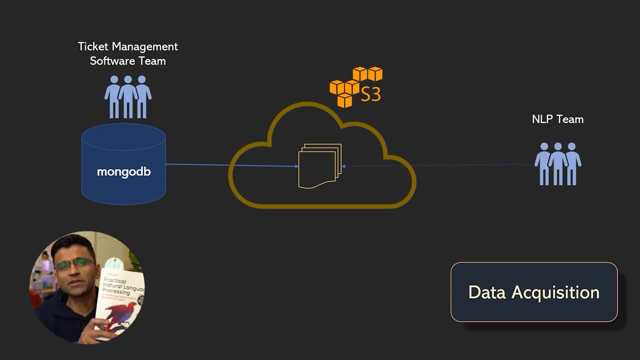 the data. I have this practical NLP book. This tutorial is based on some of the content of this book And this book has given a lot of examples on how one can collect the data. So maybe I can quickly go over some of those examples here so that you get a good idea. 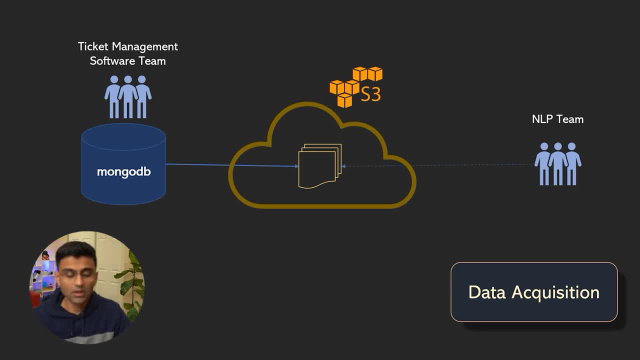 Okay, So see, some of the ways that you can collect data is: first is use a public data set such as you know, like Google has a search engine for data sets, or some of the public, like US consensus bureau website has a lot of economic data. 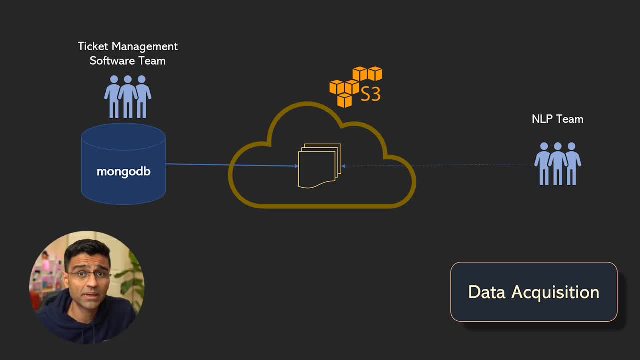 You can also use a scrapping web, scrapping and scrape the internet to collect the data. So that's one of the ways that you can collect data. Okay, So let's talk about some of the data that you need. Basically, you go to internet, write some Python script which can do web scraping. 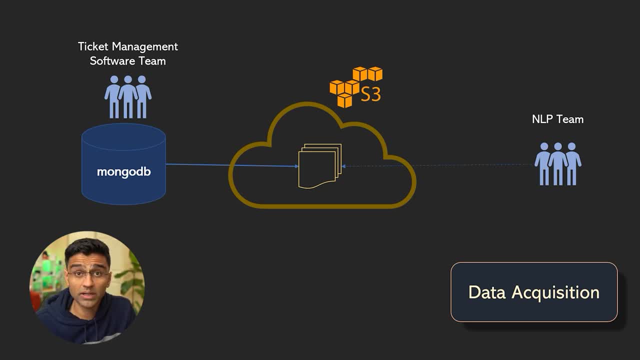 You can use product intervention. you can use data augmentation. there are a lot of techniques available in data augmentation where, let's say, you have 10 samples. out of 10 samples, you can create 100 samples. Okay, so that's step number one, which is data acquisition. 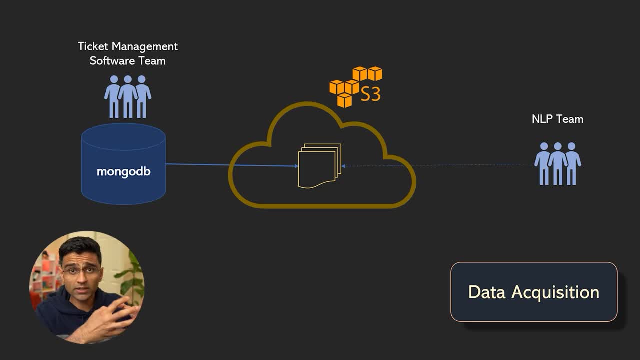 After, let's say, NLP team now got the data from NLP team. So let's say you have a S3 bucket. it's just a cloud location. you know no rocket science cloud location where you have all the records for existing tickets. 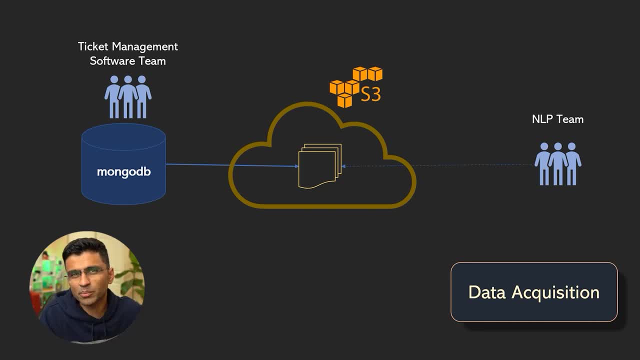 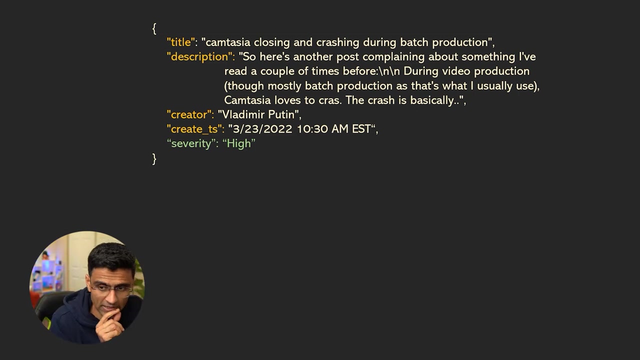 Let's say, in past, Camtasia has created 5000 support tickets along with labels, which is high, low, medium severity. all those 5000 tickets data is available on this cloud location. Now I'm looking at one record for one such ticket. 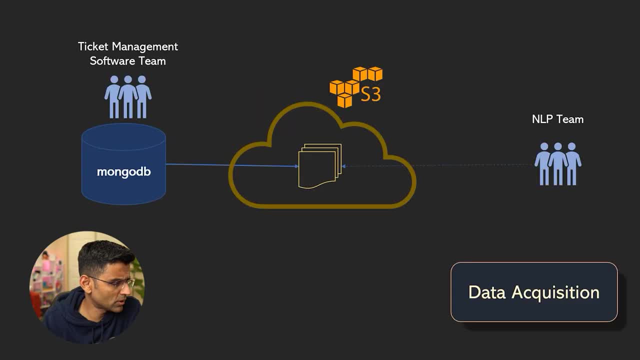 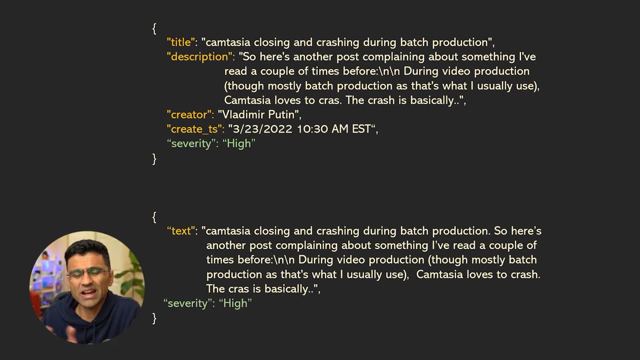 And what I can do. What I can do in this particular record is this. So I can do some. I can just discard some irrelevant information. For example: creator: create a timestamp. It's not like this ticket is created by Vladimir Putin. 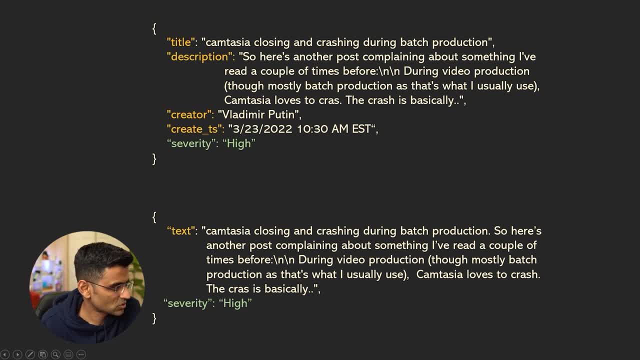 That's why I'm going to give it a high priority now. So, creator, creator, timestamp not not needed. you know this information is useless. You discard that. Title and description is something you can merge because in then you look at the words. 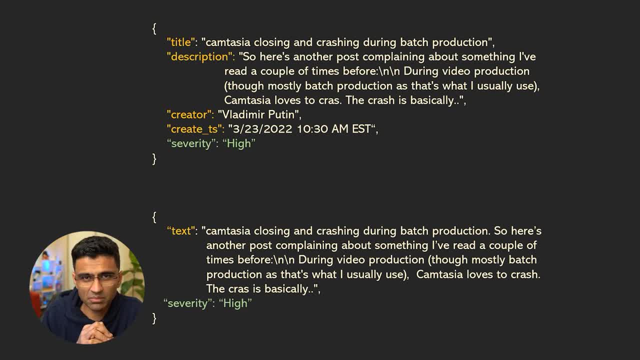 you know, such as Camtasia is crashing, for example- that's a very high priority ticket- or the software fails to render the video. So these terms could be present either in title or description. So it doesn't matter, You can just combine both of these and create a one single text. 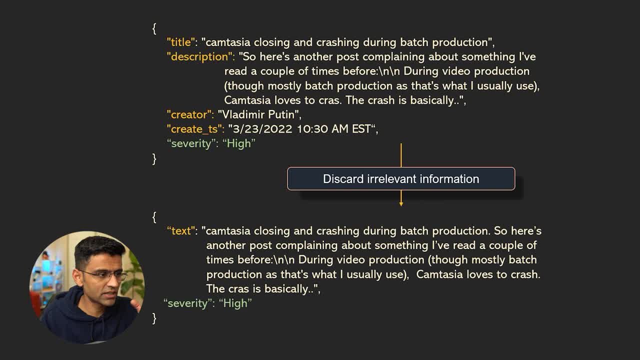 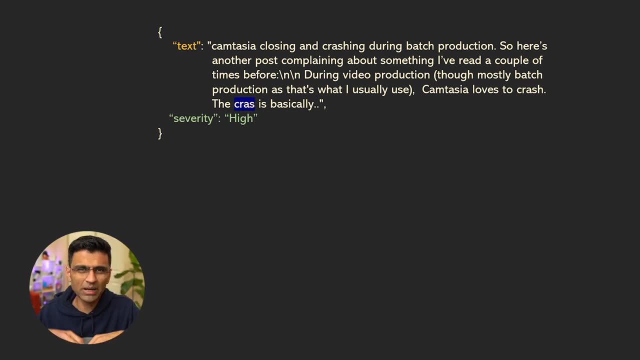 Okay, Okay, So this is what we call discarded: discarding irrelevant information and kind of creating a simple version of your text data. The second step you can do is spelling mistakes. When people enter tickets- support ticket- they might make you know fat fingering. 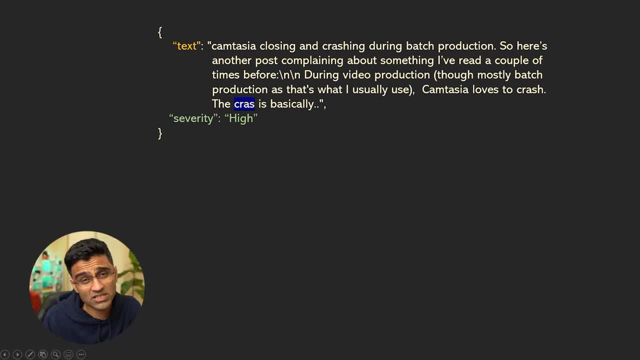 So here in this case, instead of crash C R A S H, they're saying C R A S. So you can do maybe spelling correction here. You can also remove extra slash. Slessing is like the new line breaks right. 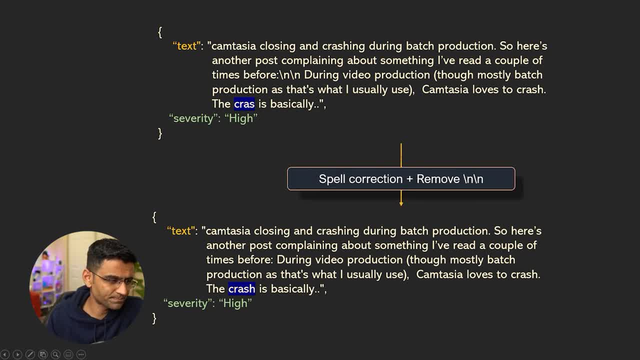 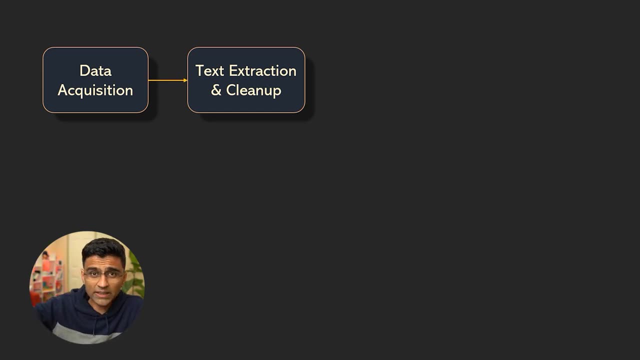 So here you see there are two Slessing, So maybe you can remove them. So spelling correction, removing those things, you know, extra line breaks, all of these things combinedly are called text extraction and cleanup. So the data that you got was very raw. 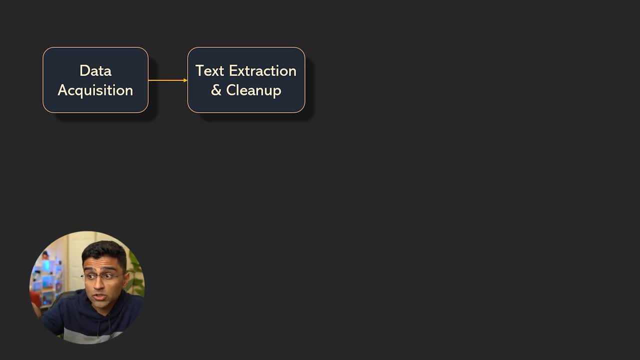 It has a lot of extra information. You did only useful information out of it And then you did some cleaning on it On top of it. Okay, So these are the first two steps in NLP pipeline. Now you have this particular text. 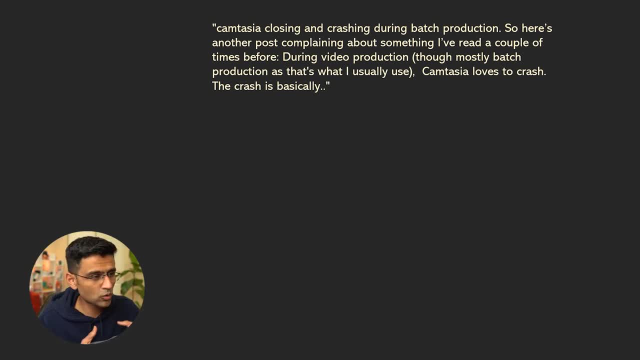 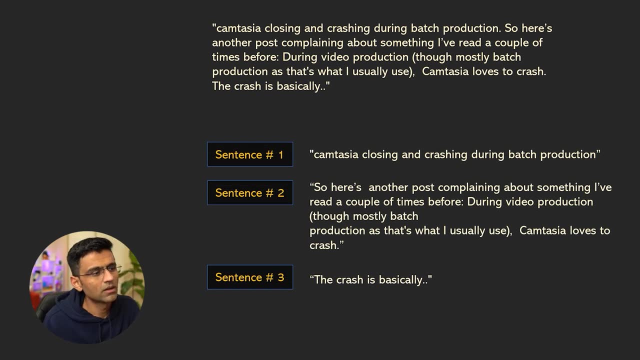 In order to build NLP model, you have to split this into separate sentences. Okay, So one way to do this is, you know, like dot, dot or question mark. that's end of the statement, So you can split it into three different statements. 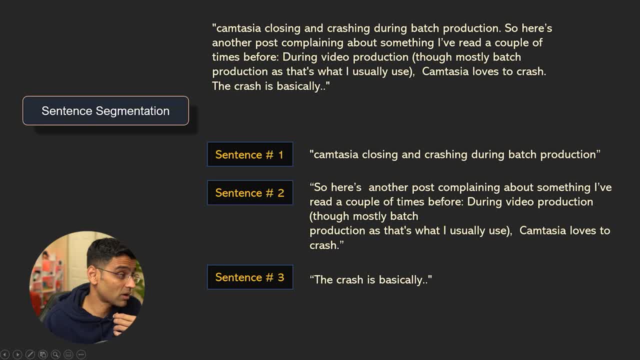 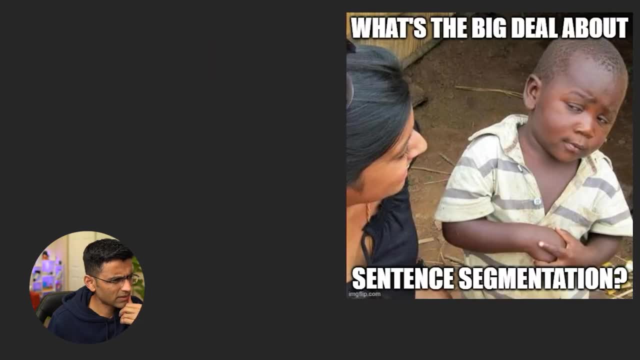 Three different statements And this process is called sentence segmentation or sentence tokenization. Now you'll be like: what's the big deal about sentence segmentation? All you do is look at the dots and question mark and you split the sentences. But look at this statement: Dr Strange likes samosas and ravioli, so that his brain works. 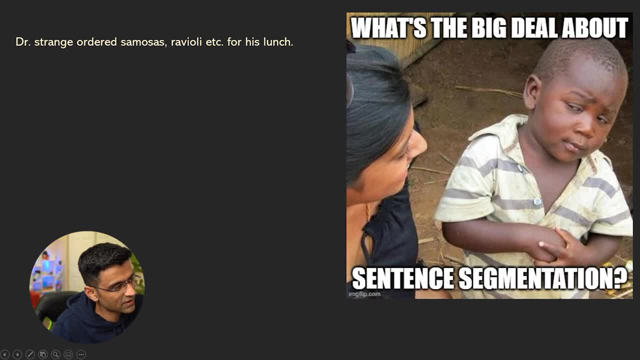 fast Now, After doctor and after ETC there's a dot. So if you just use that dot rule you will end up creating three sentences. So you see, splitting sentences is not just straightforward. You have to incorporate a lot of rules of the grammar or a specific language to build. 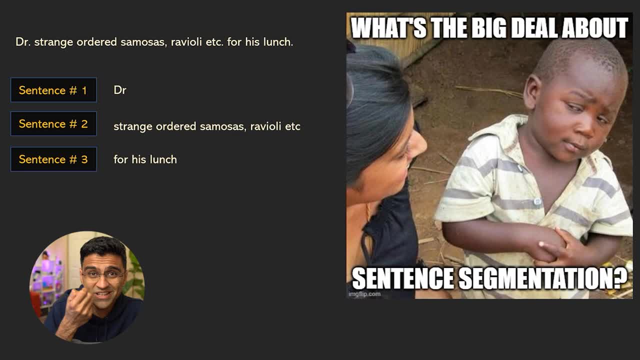 a good sentence splitter, you know, or sentence tokenizer, And the Library is like NLDK and specie has this kind of ready-made tokenizer that you can use And in the future video we will write code and we'll look into it. how those tokenizers 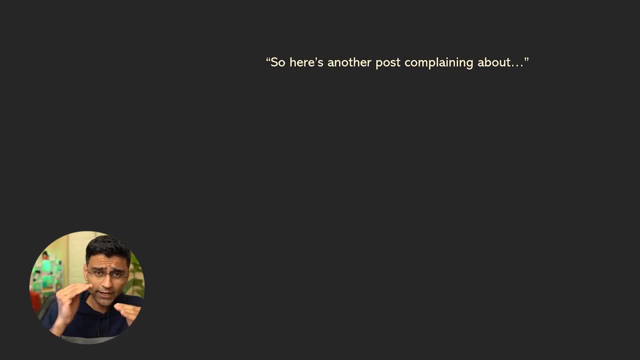 works. And once you have created separate sentences, the next step would be to create separate words. you know, and that process is called word tokenization, because once you create separate words, then you can create a machine learning model and build your NLP application. 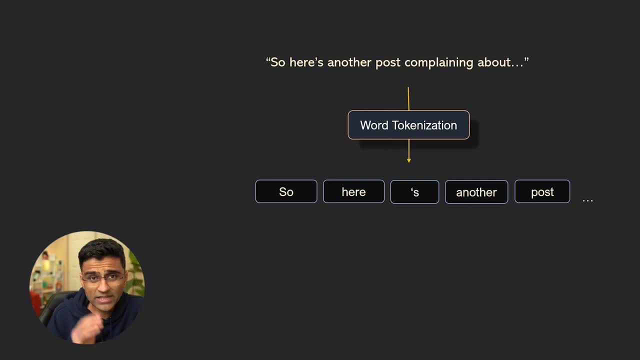 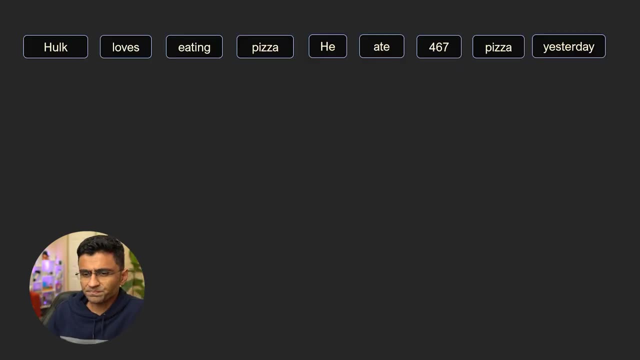 Eventually. So that's word tokenization, or sometimes people just call it tokenization. Now let's say I have from the big text blog, I create a sentences from sentences, I created individual words. Now I need to do some further processing and, you know, do you think it will make sense? 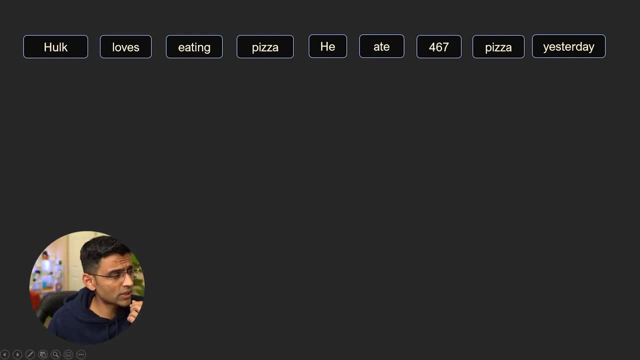 that this word eating to its base word eat, or the word loves to its base word love, because that way if someone is saying eating, eats, ate, if you can map it to its base word, then it will help you in the model building process and we'll see in the future how exactly this is helping. 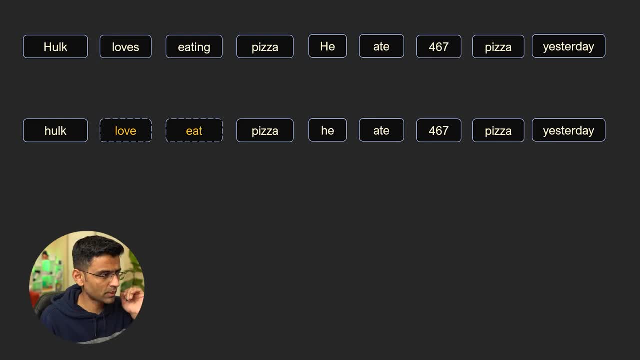 and this step of removing, for example, from eating i removed ing, so i can use some simple rules that if you have ing, remove it, okay, that kind of rule i can use and that process is called stemming. so stemming is basically using some fixed rules to try to come up with a base word. 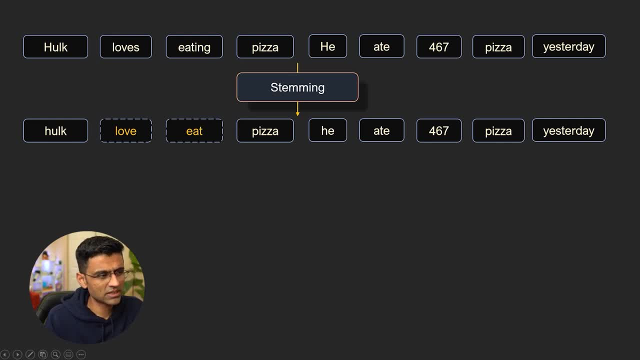 but stemming might not be the same as stemming, but stemming is the same as stemming. stemming might not be the same as stemming, but stemming might not be the same as stemming. enough, because see here, watch this word: eight, eight. i expected to map it to eat, but it's not. 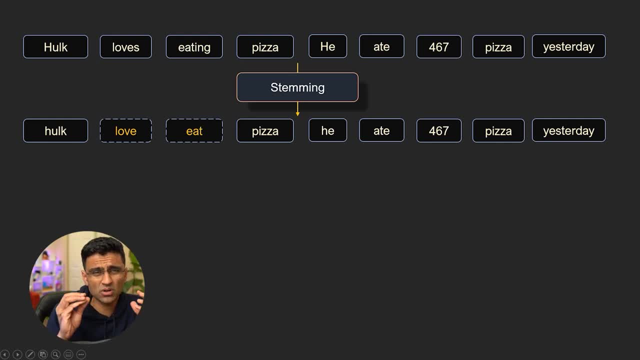 doing that because stemming doesn't know grammar, it's just based on some simple rules. so then you can use a process called lemmatization. lemmatization means you are mapping that word to its base word. so eight is a past tense of eat, so you're using lemmatization to come up with that word. so you see. 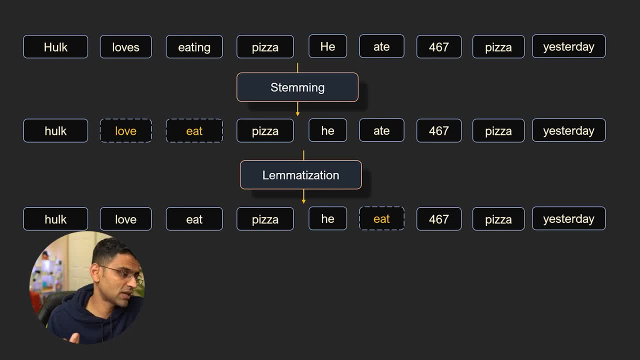 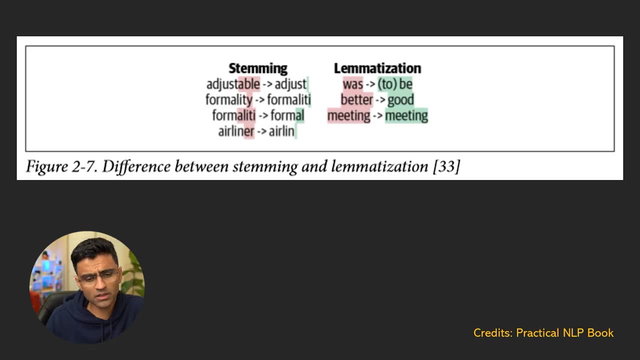 you did two phase process here- stemming and lemmatization- and that gives you the base words for each of your original word. and here is another diagram from the same book that i was referring to. the book link is in video description below if you want to order it and read it. it has a lot of. 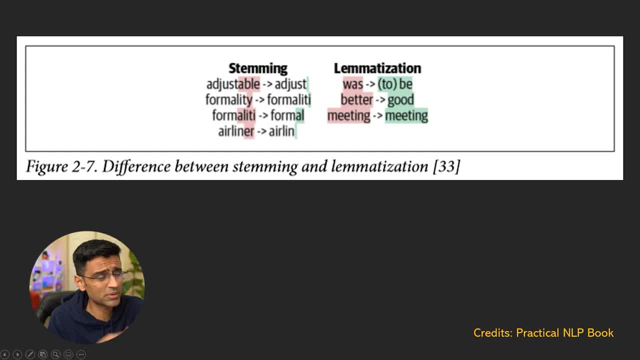 useful information, but this shows some examples of stemming and lemmatization. you see, lemmatization, if you have better, it will map it to good meeting. it will map to meeting, of course, but there is no base word here, but stemming just uses simple rule like: if you have able, it will remove. 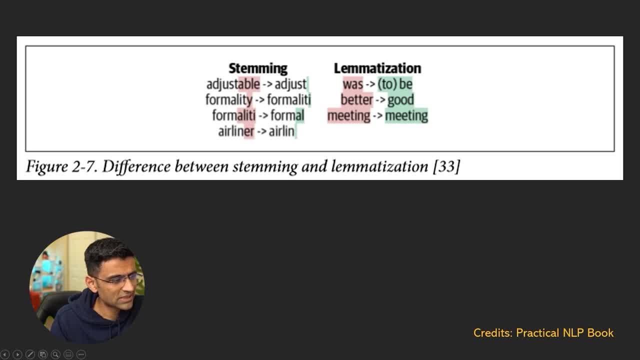 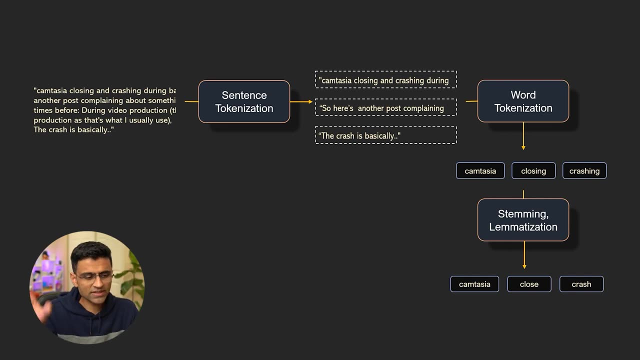 a, b, l, e. if you have formality, it will say formal. see, sometimes it might mess up some words like airline, airline, airliner, airline doesn't make sense, but it still works in practice. so this summarizes the whole process. you had a big text blurb, you created a sentence. 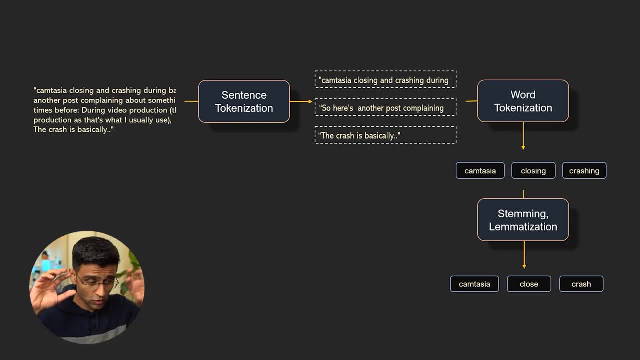 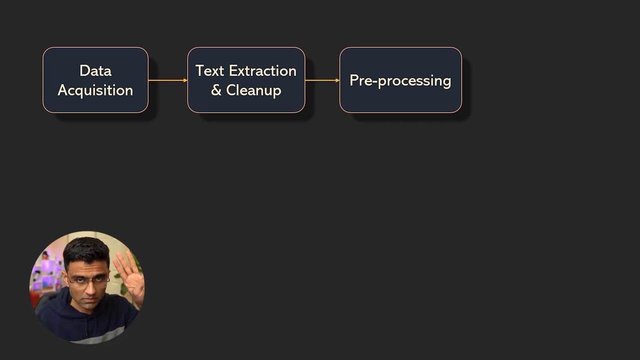 you created words and then you use stemming and lemmatization to come up with the base word. this whole process is called pre-processing. okay, so what we saw is data acquisition, text extraction and pre-processing. these are the first three steps in nlp pipeline so far. now you got all these base words. what do you do? see? you are trying to create again what is. 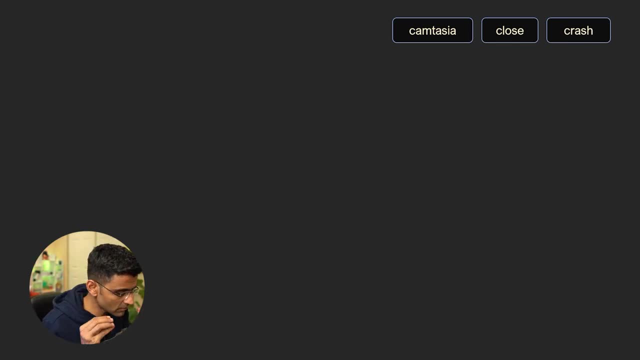 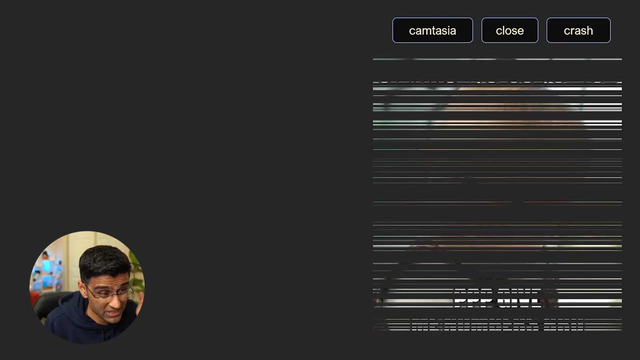 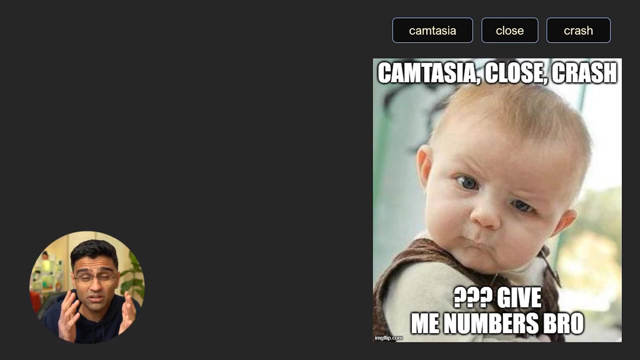 our end goal and goal is to create in a classifier that can take the text of support ticket and it can tell me if it's a high priority ticket or not, or low priority, etc. now i got all these words. machine learning models do not understand text. they always ask for numbers. so what you can do is you can use some formula, some technique. 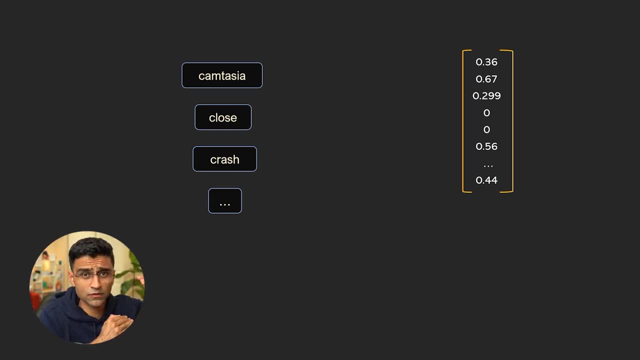 so that you can convert these words into numbers. now, what kind of numbers again, we'll see that in the future, but some meaningful representation of these words, such that similar words you know, like feeling better versus feeling good, these words will have similar number representation. then my model can work better. 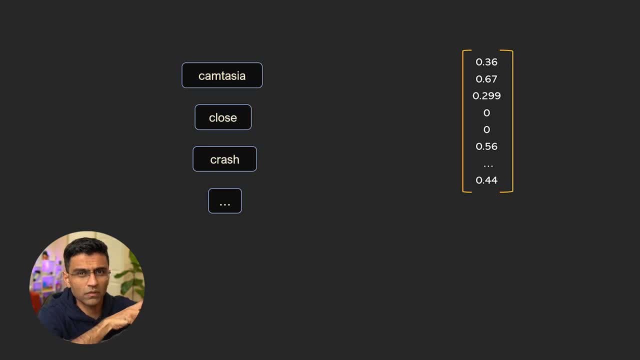 and, and this process of converting words into number is called feature engineering. feature engineering is you are extracting features from that word. if you have a word, good and well, then there are certain features. you know, if you have, let's say, a cricket player name, dhoni versus whatever, dhoni versus, let's say, 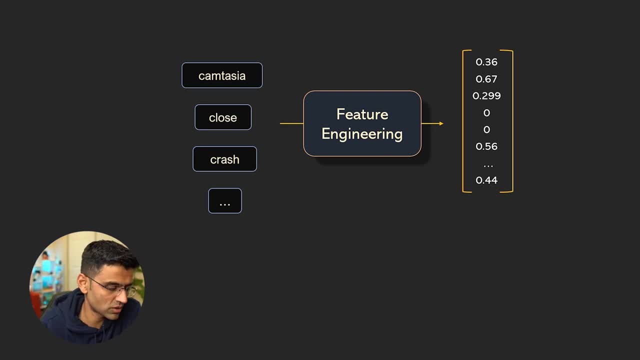 ricky ponting or shane warne- he died recently, unfortunately- these, if you want to represent these words or person in in a vector, you can have different features, such as: okay, is this a sports player one or zero? is this a human one or zero? because if i have, you know, if i have a bottle, bottle is not a human, so you can have this kind. 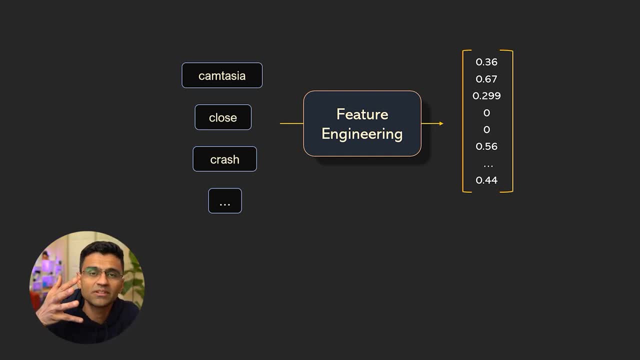 of features and this feature vector can represent that word in an appropriate way. and that technique of extracting features is called feature engineering. and there are various popular techniques. i'm just going to throw different jargons, don't worry. tf-idf, factorizers- one hot encoding word embedding. we'll cover all of that in the future videos. 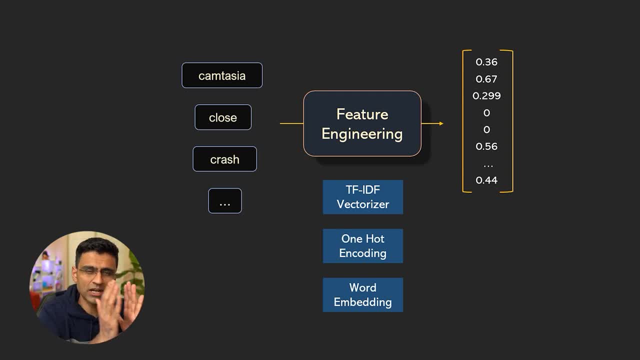 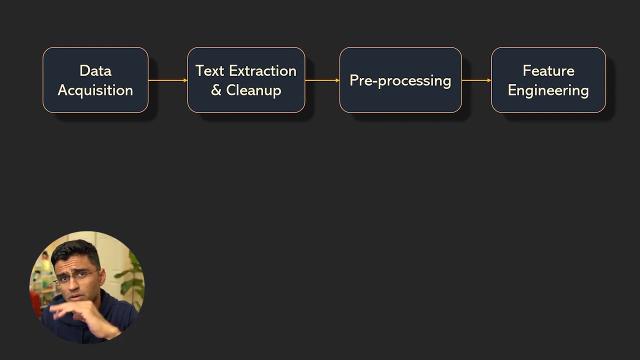 but just for now, just assume there are some good ways of converting words into numbers so that these numbers present this word in an accurate way. okay, so so far we have seen these four steps. once you have done feature engineering, your next step will be to build machine learning model. not all nlp applications require machine learning model. 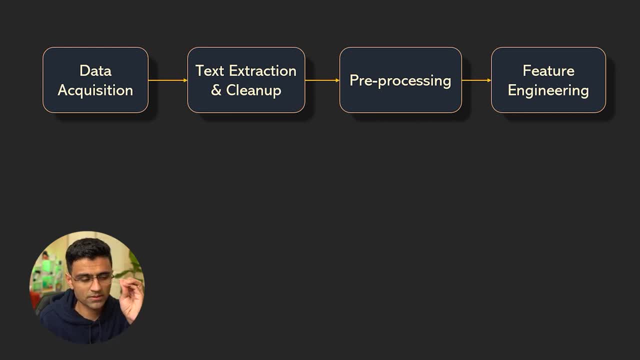 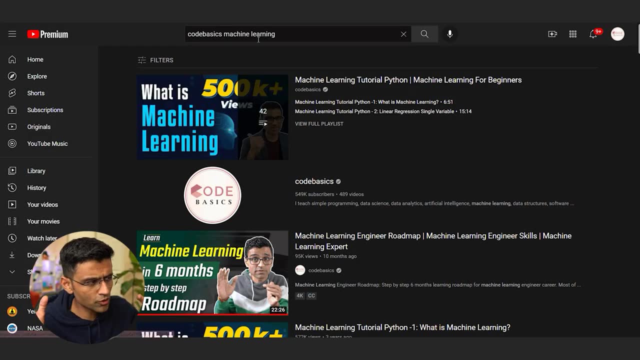 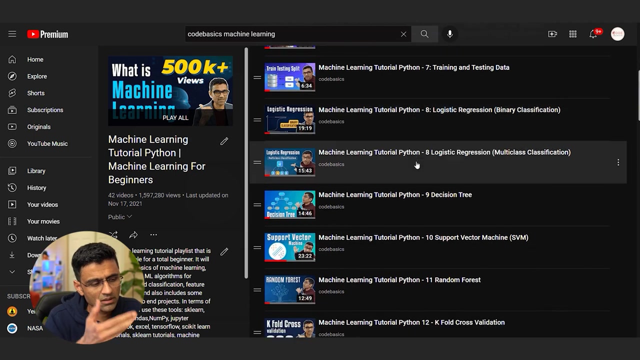 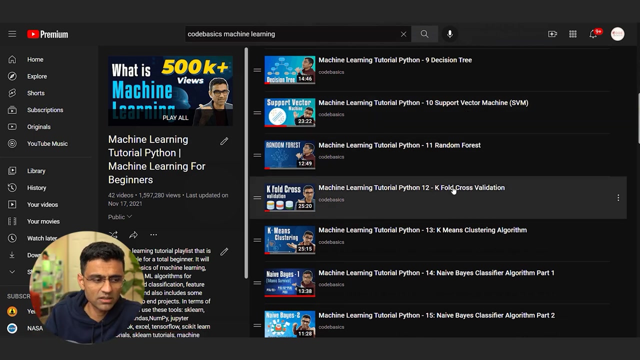 but the one that we are talking about support ticket. classification using machine learning might be useful here, so go to youtube search code: basics machine learning. you'll find my tutorial playlist and in this playlist there are various classification techniques, such as decision tree, see support vector machine, random forest. all of these are various classification techniques. 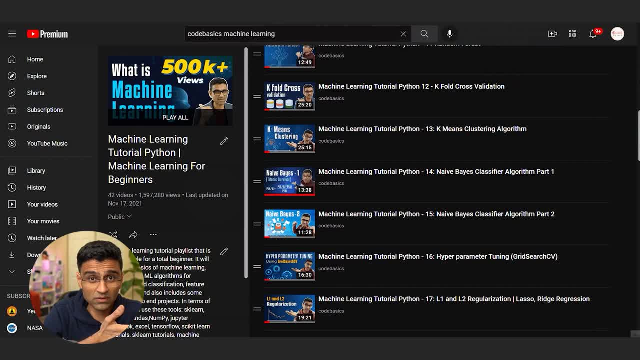 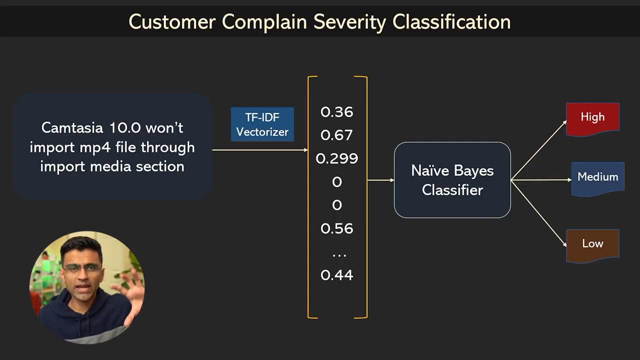 naive base, so it will be useful. if you go through this ml playlist, it's going to help you. all these classification techniques can be used for our problem. so let's say for our problem. we end up using naive base. so you had support ticket text. you somehow converted it into numbers for now don't. 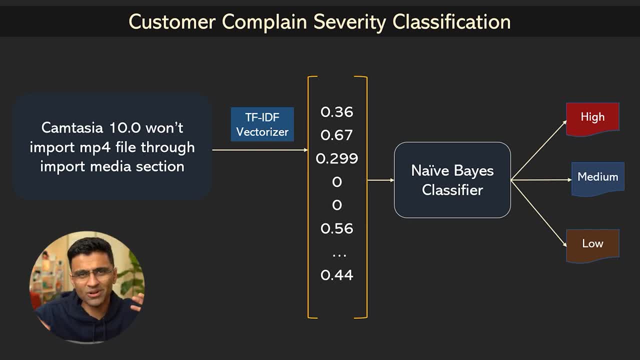 don't worry how we convert it into numbers, but machine learning model understands numbers. that's why we converted it into numbers. and then we use naive base classifier, let's say or svm or any other classifier, and we can do classification. so if you have 5000 support ticket data in the past, 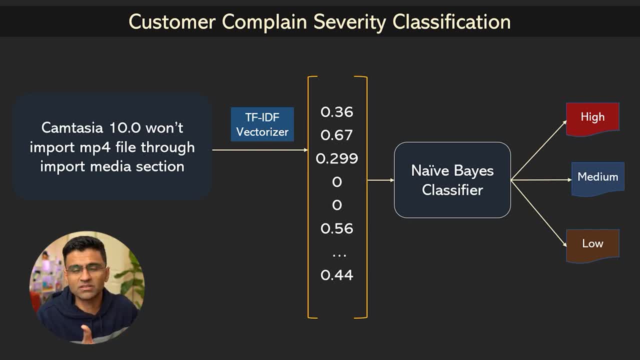 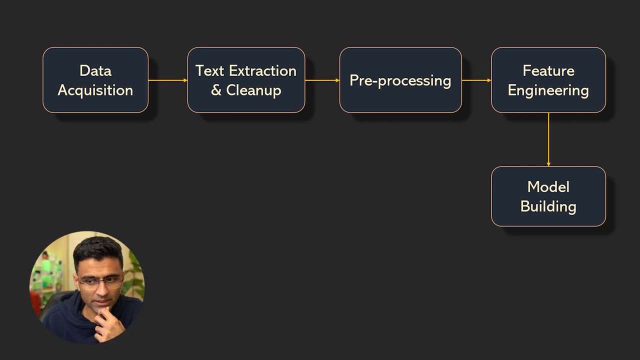 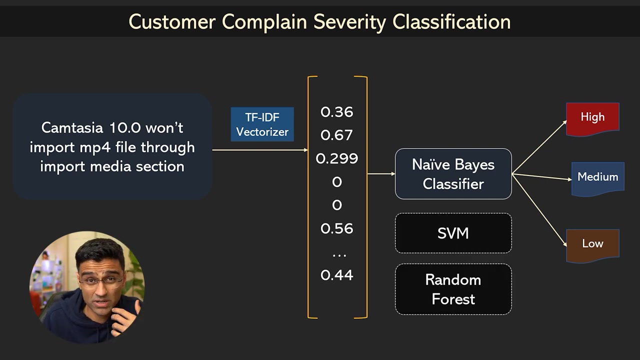 along with the labels. now we can train this model with that data and in the future, when the new ticket comes up, when you feed it to this model, it will tell you whether it's a high priority or low priority. so that was model building. now, as i said, you can use different techniques: svm, random forest and within specific. 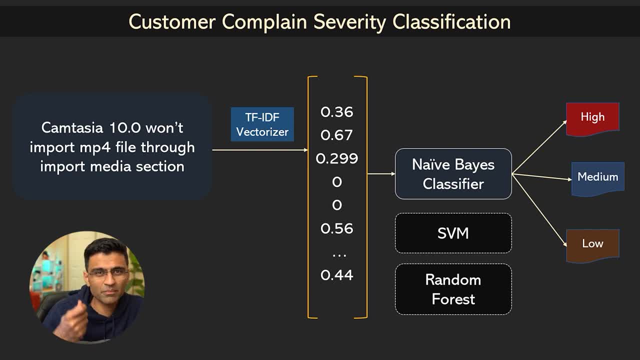 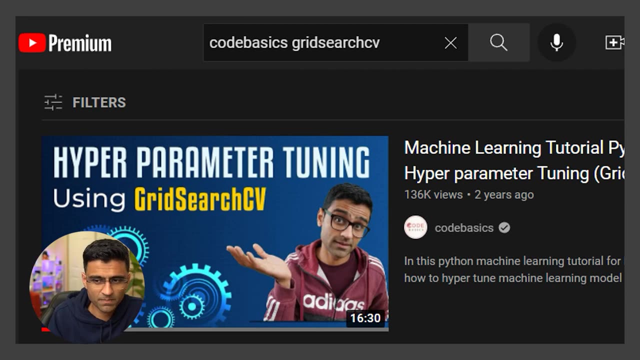 technique. also, there are hyper parameters. there are different parameters, like cog wheels that you can tune, and to figure out which model is the best model, you can use a technique called grid search cv. again, go to youtube. i have a video on this. you can watch that. but these kind of techniques allow you. 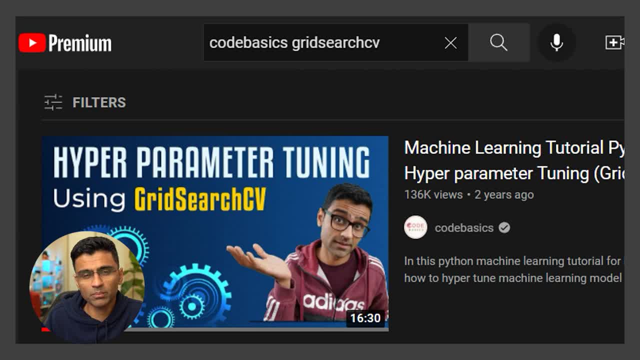 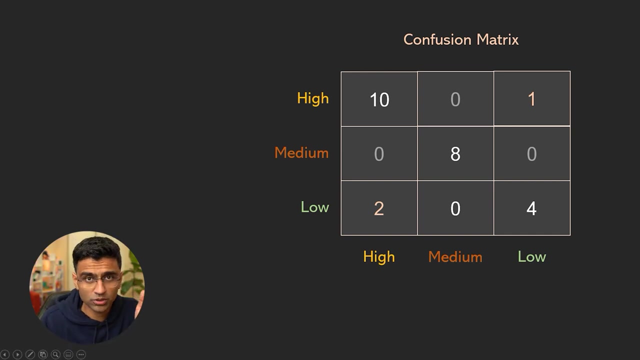 to choose the best model for your given problem, because model building is short of like file and error. you have to try a lot of things and eventually something works. you know it sometimes, yet know without doing anything. the results don't always think that way. okay, now, when you are evaluating your model, you can use something called confusion matrix. 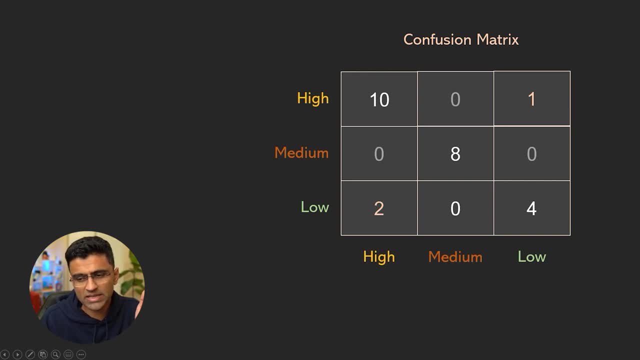 so in confusion, matrix on the x-axis, you have truth, this is truth and this is prediction. so let's say, i built a model, after that i started predicting and so in conclusion, when i build the model, then what will happen? after that i start to predict, i can start to calculate that. predictions that may be看一下 and activation pattern and fragments, but this is where you get the rightnext contributionHypoth instincts over, because it's not evaluation model. it's for this reason i am going to use right now and for this reason i am going to change the order in one point in between, i'm just going to say�. 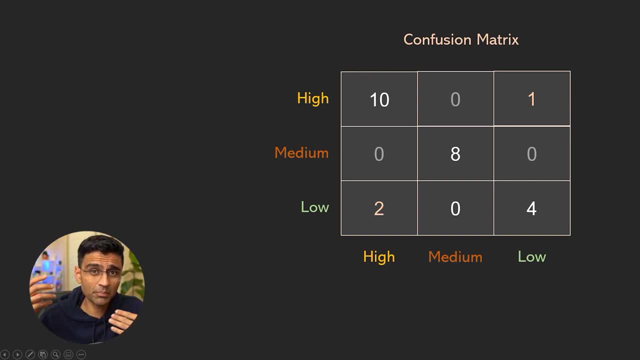 So when I do the prediction, I can then compare it with the truth and I can figure out how good my model is. So let's say, in this test there were 10 tickets, which was actually high priority, and my model predicted it to be high. 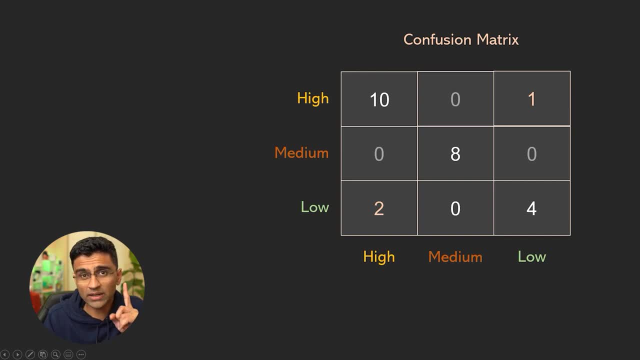 So anything on this diagonal is. I got the right prediction. So there were eight tickets which were medium priority and my model predicted it to be medium. But look at this too. So there was two tickets which was actually low priority but my model said it's a high. 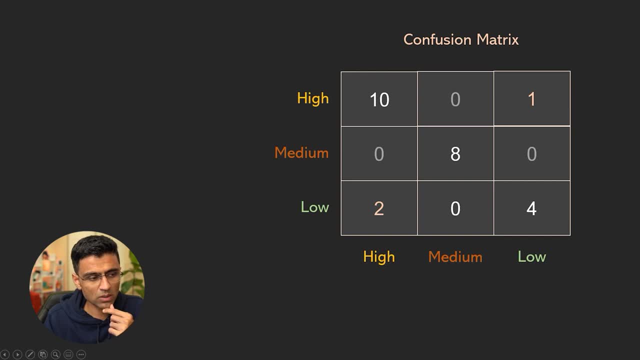 priority. So anything that is not in this diagonal is your wrong prediction. So you can, by looking at confusion metrics you can figure out how confused your model is. It's like if your model is not confused and very accurate, then you see all the numbers. 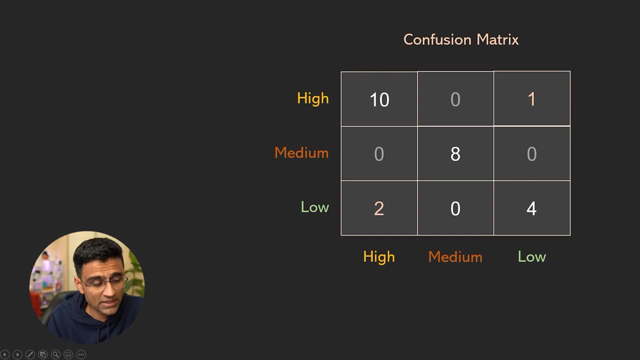 in the diagonal and everywhere else You will see zero. In this particular case, two and one three, it made total three, wrong prediction. And when you are building machine learning model, you can use different metrics like accuracy, precision, recall, F1 score to figure out if the model is good or not. 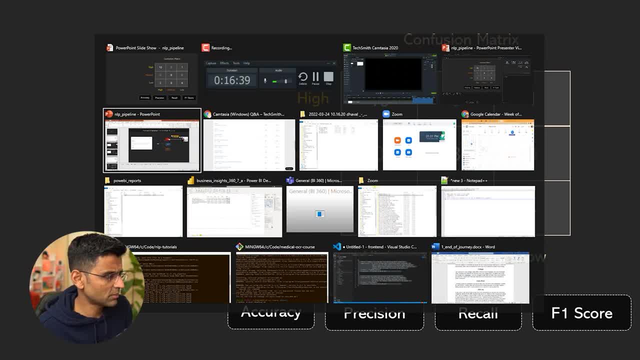 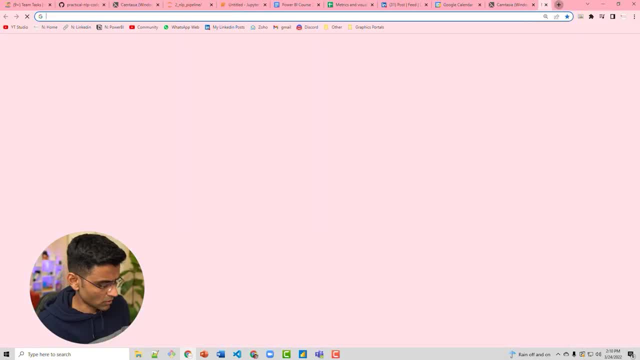 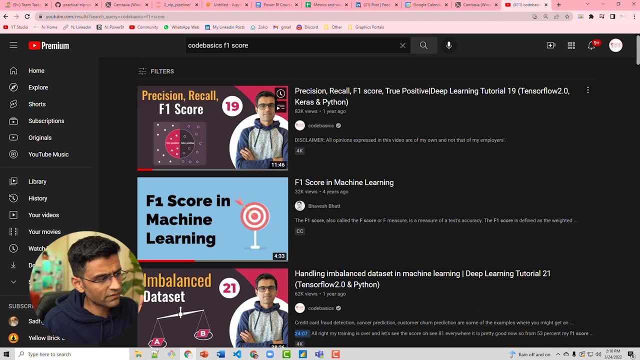 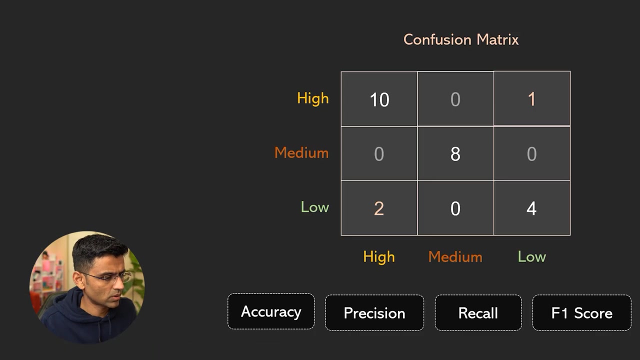 If you want to know precision recall, F1 score, et cetera, Let me suggest you A. So if you go to YouTube and if you search for code basics, F1 score, you'll find a video. This video will give you a very good, simple explanation of precision recall and so on. 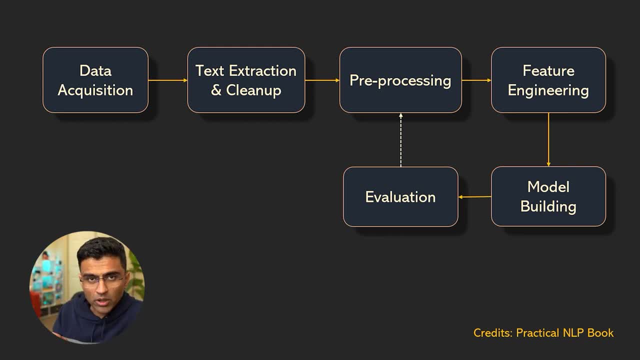 Okay, So we build a model, we evaluate using grid search, CV, confusion metrics, And if things don't look good, we again, we kind of go in a loop. you know, this dotted line shows You might have to do revisions. 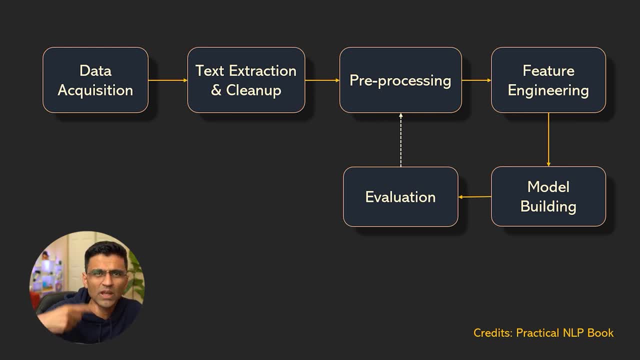 You might have to do again pre-processing, feature engineering, model building. You keep on trying, iteration, until you find a perfect model for your problem. I mean, there is no perfect model, but a model that performs better than others. Once a model is built, you can export it to a file and deploy it on the cloud Azure. 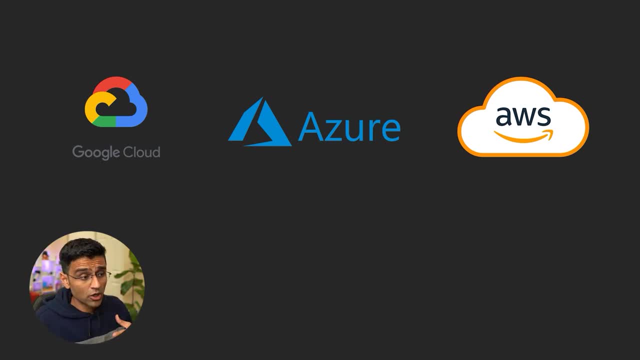 Google cloud, anything, AWS. You can write a fast API base Or fast text service around not faster fast API or flask service around that model. So there is a model and you can write a risk to service. you know the HTTP, the service. 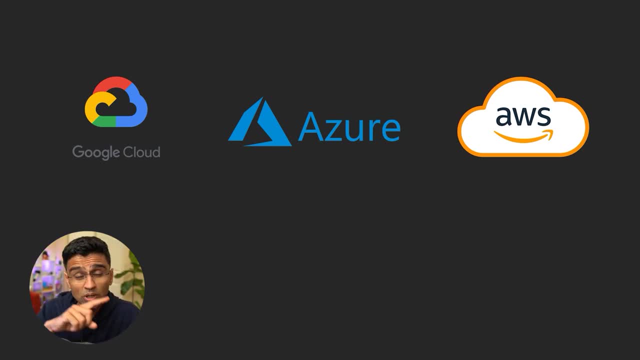 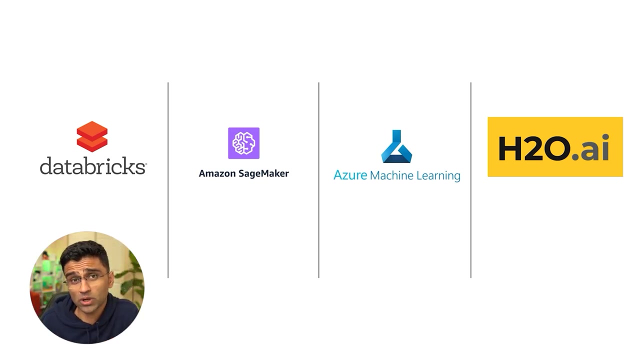 that can request as so to HTTP request. You can build that service and you can deploy that service in the cloud. You can also deploy it to an end to end ML platform, such as Databricks, Amazon server, Amazon server, SageMaker, Azure machine learning, H2Oai. 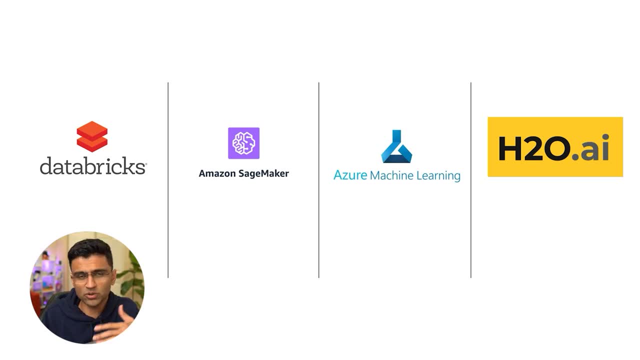 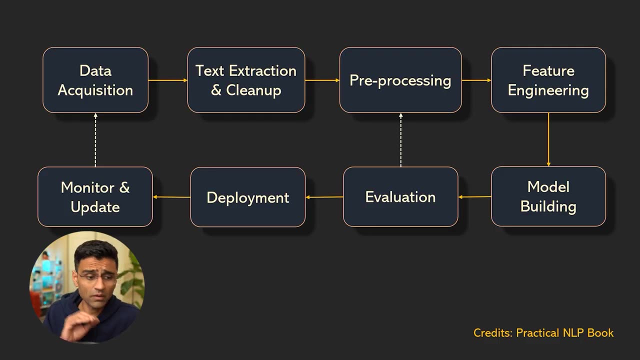 These are like end to end machine learning platforms that you can use to build and deploy these services. And once the service is deployed- of course you do- you do need to monitor and update it periodically. When you deploy it in production, when it starts serving requests, you have to set up 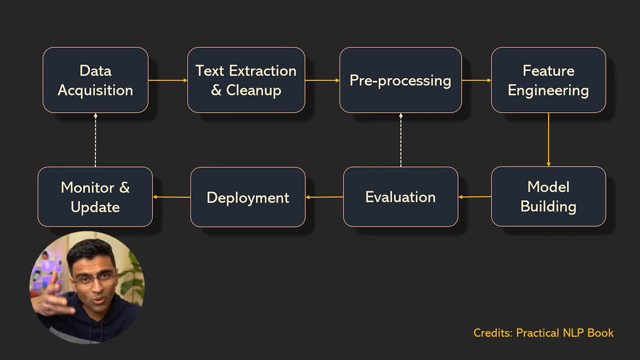 some kind of monitoring system so that you know, Because sometimes In the dev things work OK, but when you deploy to production, when the model goes in wild, maybe it doesn't perform as good. So having a good monitoring and update system make sure that you know the model is not doing. 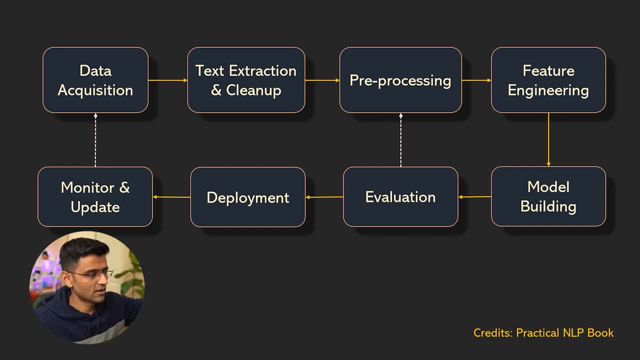 wrong prediction and you're not losing on your business. And there is a dotted line here again means if the model is not performing well, there are n number of reasons. Let's say there is a drift in the concept. We build a model on specific terminology. 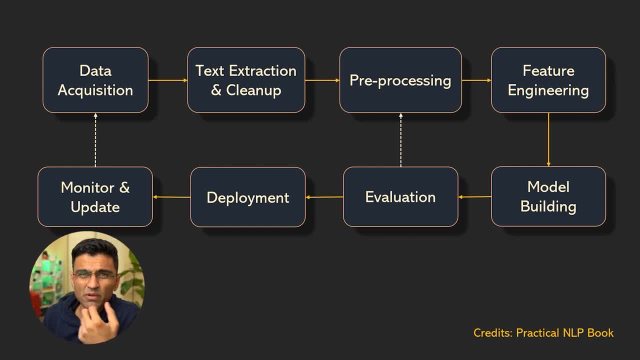 Now, let's say, companies added a bunch of new features and the way people talk kind of changed. You have to now get more training data and kind of repeat the whole process right from data acquisition to model building. OK, so understand that in the industry when you're working on NLP application it's not. 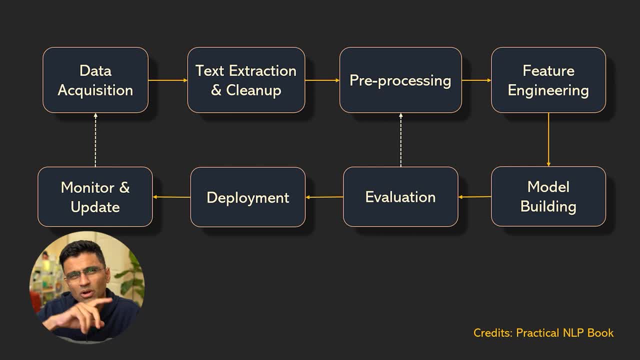 like you, build a model, deploy it and done. It's continuous iterative process. A lot of grunt work, Right, A lot of grunt work- that goes into building an NLP system. This particular conversation gives you an idea on specific use case, which was